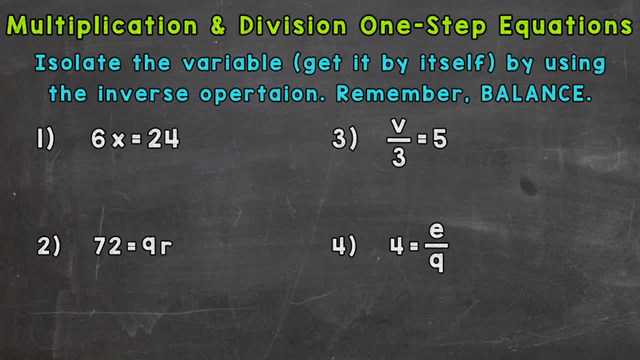 So at the top of the screen is a very important note. We need to isolate the variable, get it by itself by using the inverse or opposite operation, And always remember balance. So let's see exactly what that means as we go through our four examples. 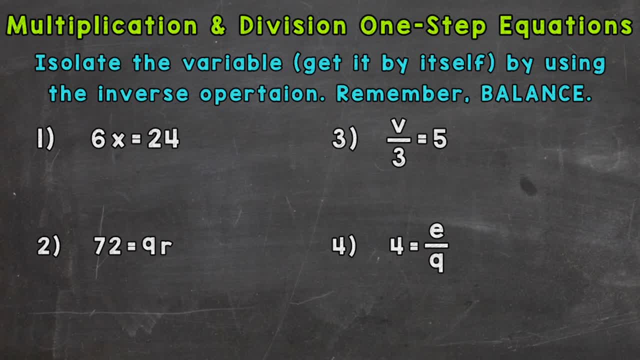 And we'll jump right into number one, where we have: 6x equals 24.. So we need to isolate that variable. We need to isolate that variable of x Now, whenever we have a number right next to our variable. so the 6 right next to the x, that means to multiply. 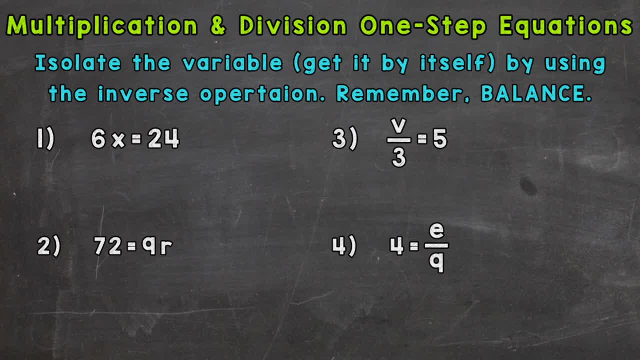 This problem means 6 times x equals 24.. So if we're multiplying by 6, the inverse or opposite operation would be to divide by 6.. So let's divide the left side by 6 in order to isolate the x, because these 6s are going to cancel out. 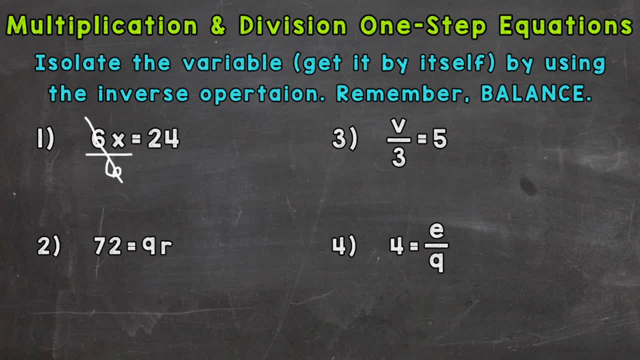 so to speak, 6 divided by 6 there gives us 1x, which we can just write x there, and we have it isolated. Now, remember, we have to keep everything balanced. So whatever we do to one side, we have to do to the other. 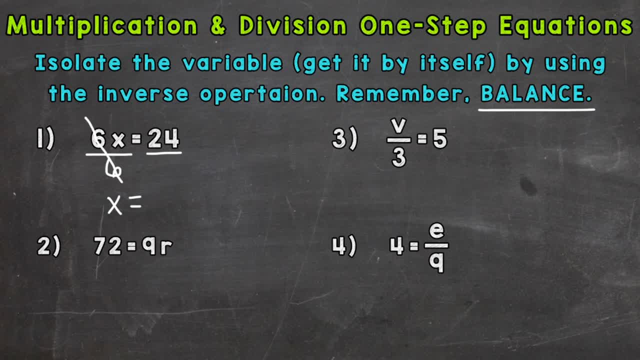 So if we divided the left by 6, we have to divide the right by 6.. So 24 divided by 6 equals 4.. And we have our answer: x equals 4.. Now we can always double check our answer by plugging it back in to the original equation. 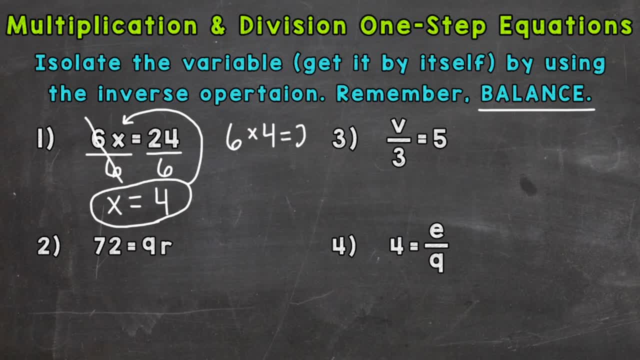 So 6 times 4 equals 24.. That is true. so we have the correct answer. Now on to number 2, which looks a little different than number 1 because we have the 72 on the left and the 9 times r on the right, so the variable is on the right. 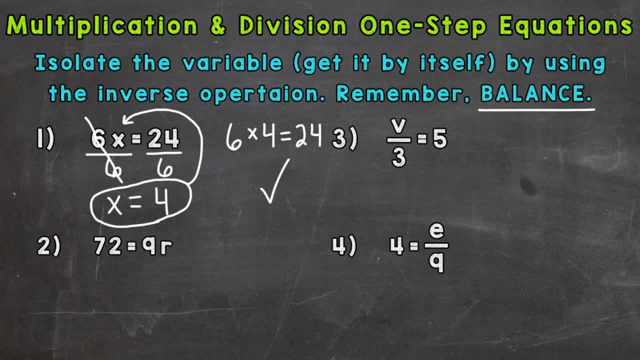 But we use the same exact process, So we need to isolate the r. We're multiplying the r by 9, so the opposite would be dividing by 9.. Now those 9's cancel out and give us 1r, which we can express by just writing the r by itself. 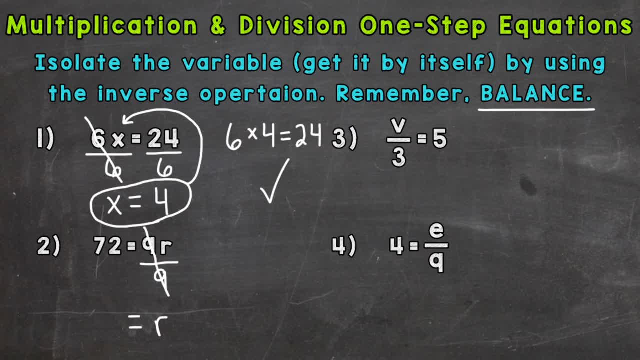 So the r is isolated. Whatever we do to one side, we have to do to the other. So 72 divided by 9 equals 8.. So we're left with r equals 8. and we can plug back in here to see if this is true. 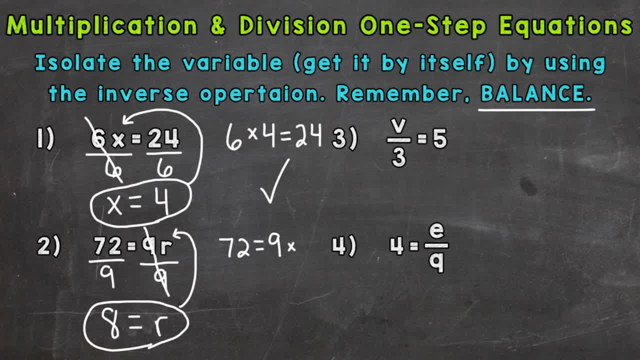 So 72 equals 9 times 8,, which is true. You can think of these equations like balancing a scale: Each side has to be exactly equal. So the left we have 72, and on the right we have 9 times 8,, which is also 72. 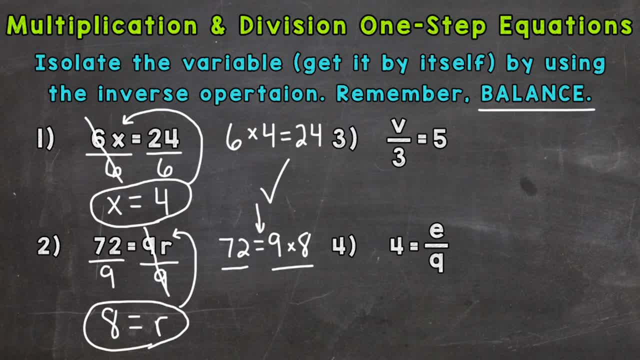 So these two sides are equal. Moving on to number 3, we have v divided by 3 equals 5.. So let's isolate the v. We are dividing it by 3, so the opposite would be to multiply it by 3.. 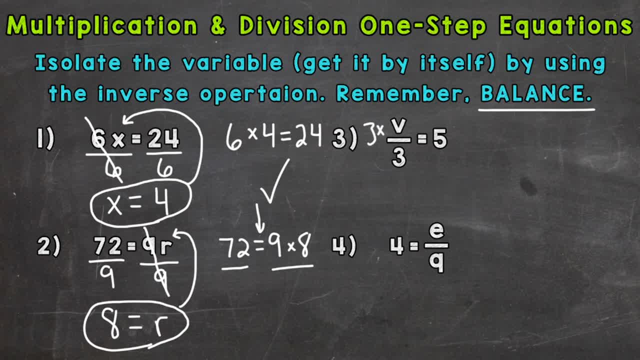 So let's multiply the left by 3 and the right by 3.. So these 3s cancel out here and we isolated the v and 5 times 3 is 15.. So we get to v equals 15. And we can plug back in to make sure. 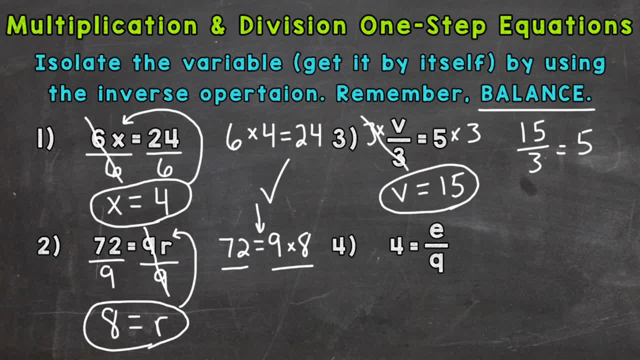 And we are correct, because 15 divided by 3 equals 5.. And lastly, we have number 4, where we have 4 equals e divided by 9.. So we need to isolate the variable of e. We are dividing it by 9, so the opposite would be to multiply that side by 9.. 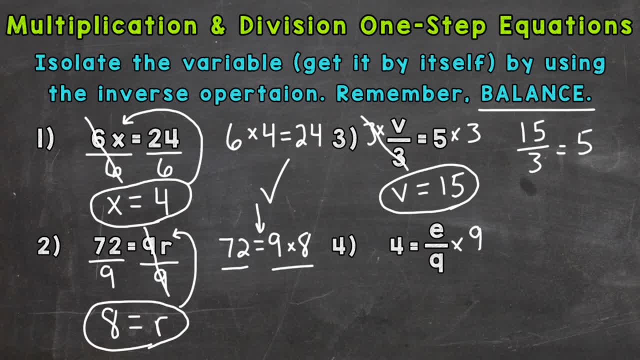 And whatever we do to one side, we have to do to the other. So multiply both sides by 9.. These 9s cancel out and we are left with the isolated e, And 9 times 4 gives us 36.. 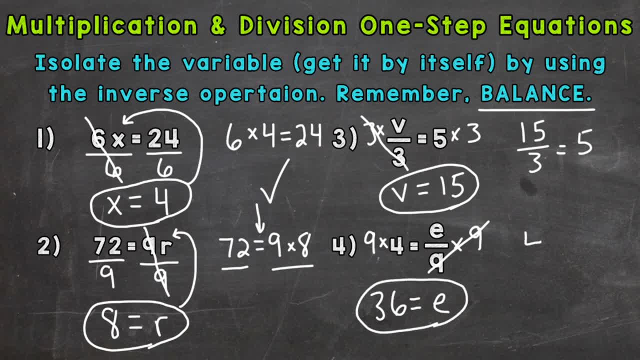 So e equals 36.. And we can double check here. So 4 equals 36 divided by 9.. Both sides are equal. So we have the correct answer for the value of i. So we have the correct answer for the value of i. 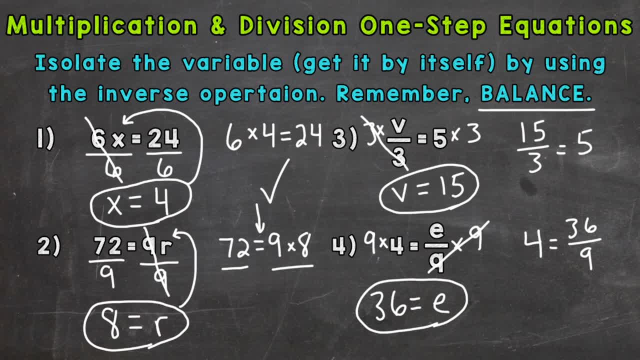 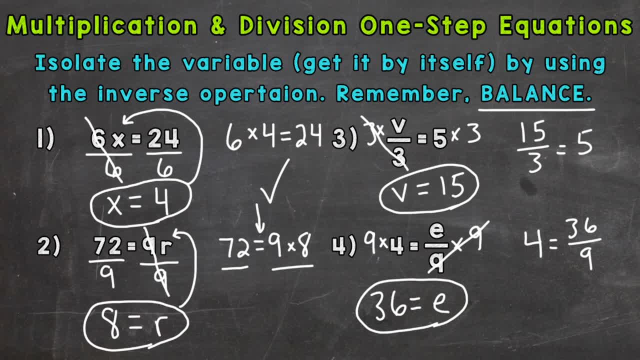 There's how you solve multiplication and division one-step equations. I hope that helped. Thanks so much for watching. Until next time, peace.